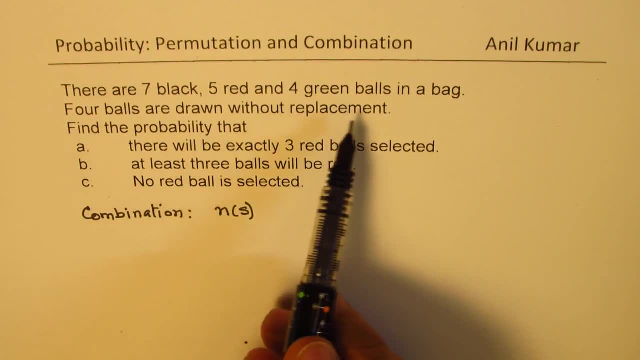 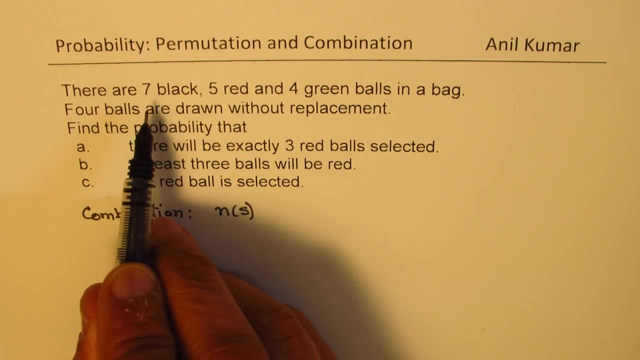 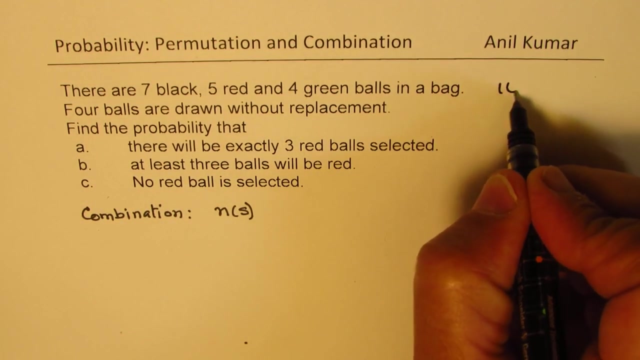 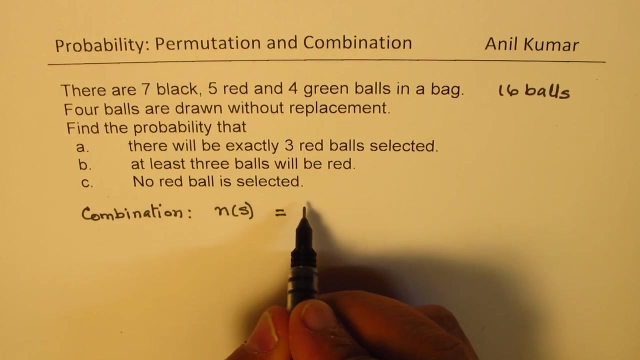 selecting four balls right from seven, five and four balls right, which is total of seven plus five is 12,. 12 plus four is 16.. So we have total of 16 balls right. So total number for us will be selecting out of 16.. We are looking for a combination of four different balls. 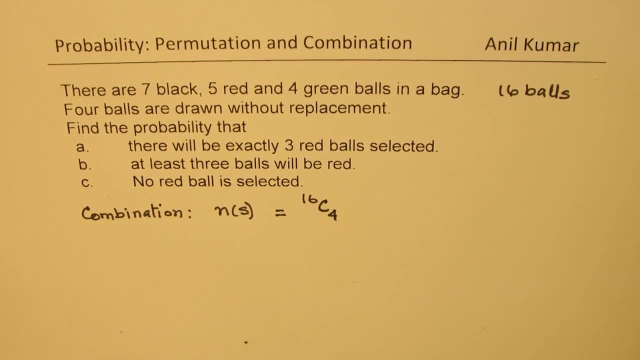 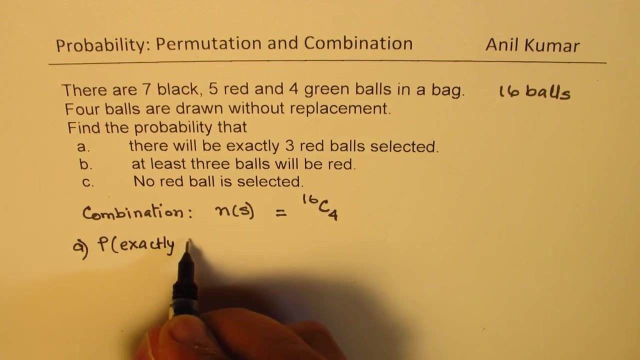 So that becomes total. Now in part A we're looking for there will be exactly three red balls, So probability for exactly three red. So red is being selected out of the five available. So when we select three out of five then it is a combination. We are selecting three out of five which are red. the others could be either black or green, which is 11, right. 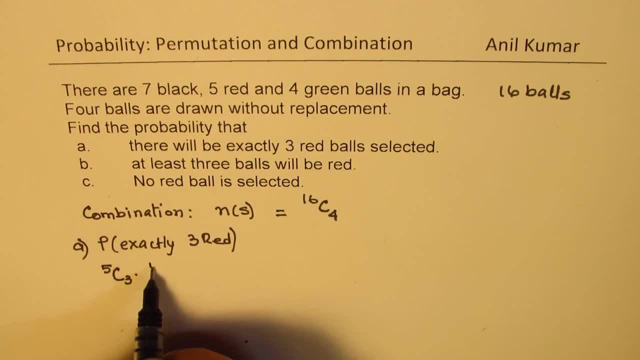 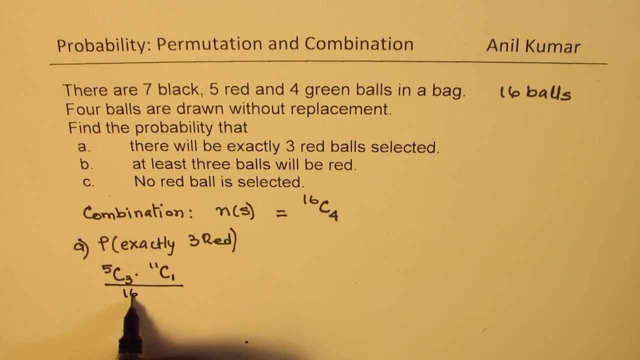 Seven plus 411.. So, out of 11, we need to select 1, divided by total, which is 16C4.. So that gives you the answer for Part A. Now, as far as part A goes, we need to divide it by 16C4.. 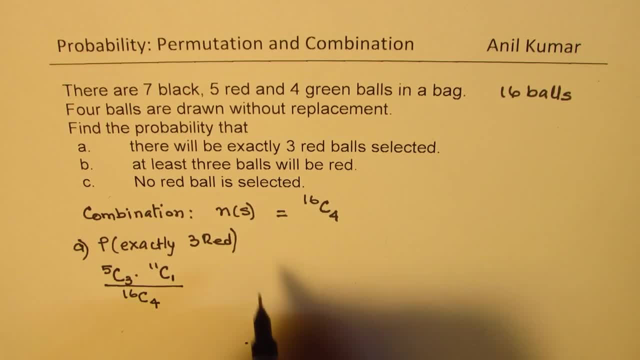 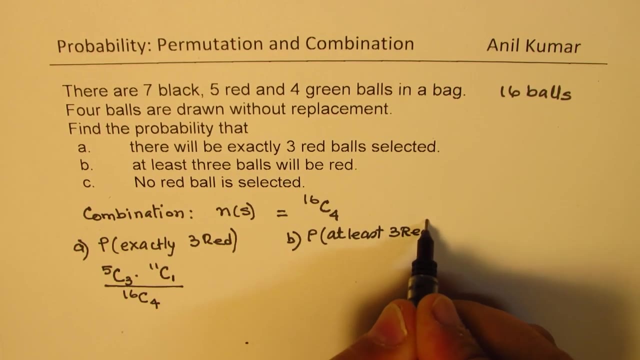 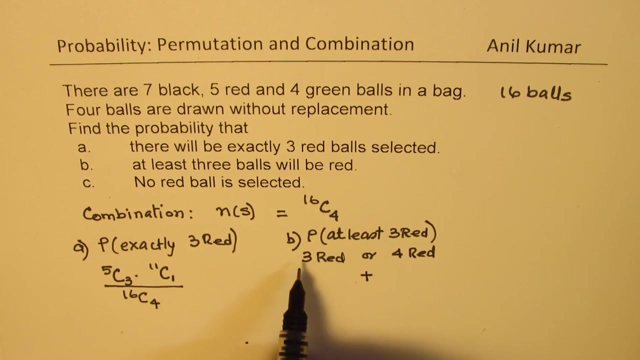 So that gives you the answer. for Part A, be is concerned, we want at least three balls will be red. so probability where we says at least three red. now, when you say at least three red, it basically means that there could be three red balls or four red balls. so that means three red or four, all are red, or means addition, right so? 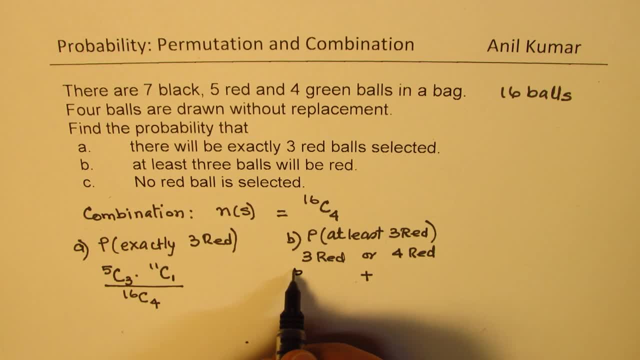 three red balls is what we have already seen: five C, three, eleven C one. all four means out of five we are selecting all four red and remaining eleven we select nothing. zero, okay, divided by total numbers, which is 16 C 4, right part C is no red ball. 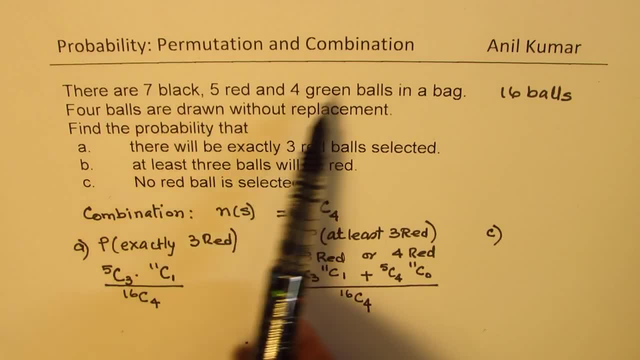 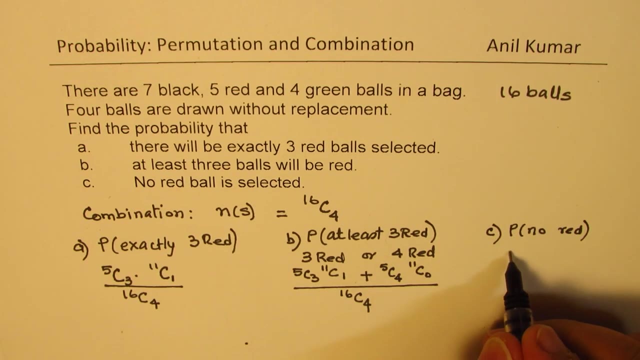 is selected, that means all the balls are selected, are either black or green right, so probability: no red. so no red means all are selected from seven or four right, so that means we have 11 as the combination for correct all right, all not right. okay, so we could. 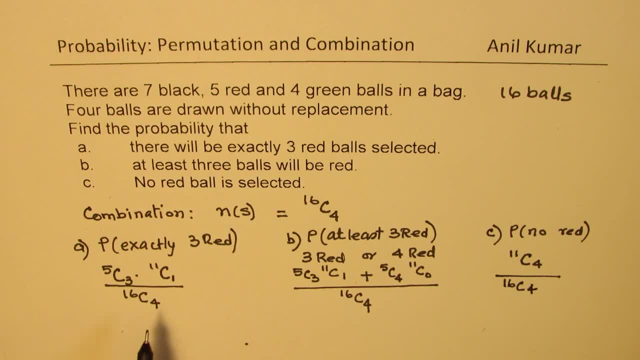 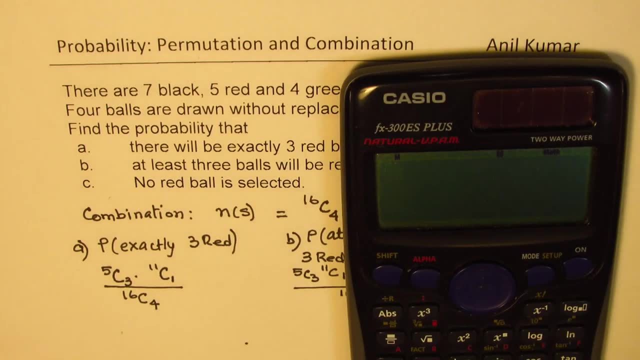 divide this by 16, C for the total number of combinations, so that becomes the answer. now many of you will be allowed the use of calculator. so if you are allowed the use of calculator, it's a very simple calculation. we can use the calculator for calculation of all gem. 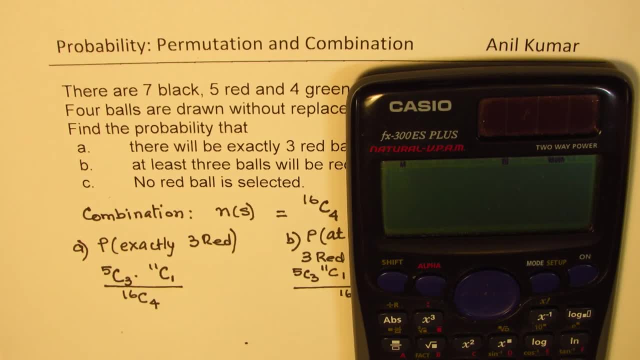 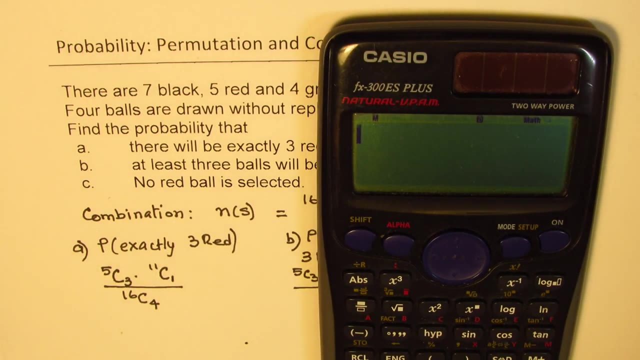 calculator get the answer. some of you may not be allowed calculator, so we will also see how to calculate these values without calculator in this video later. so let's first figure out the answers with the calculator, right? so we have 5 combination 3 times 11 combination 1. so that's the numerator and we are going to 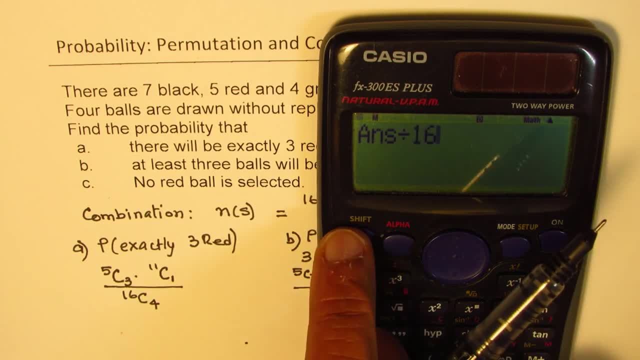 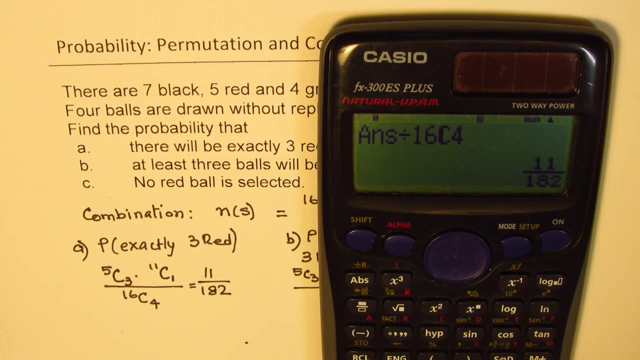 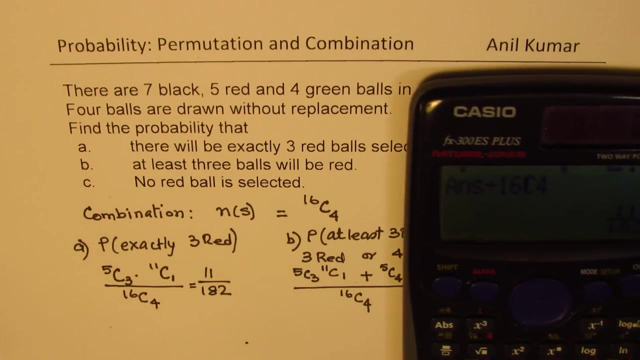 divide this by 16, combination 4, so you get the first answer as 11 over, so we get this answer as equal to 11 over 182. okay, so the next one here is now. let's do this next one: 5 C, 3, so first part is same. let's do it so we have 5 combination. 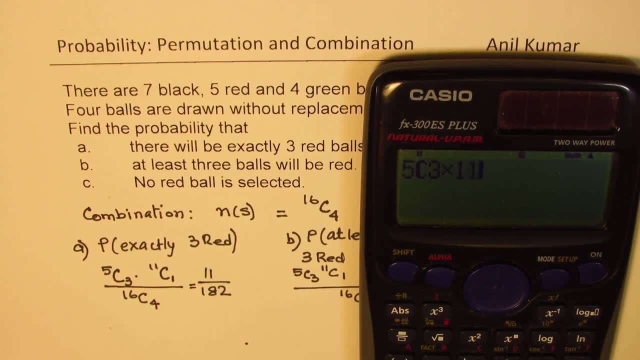 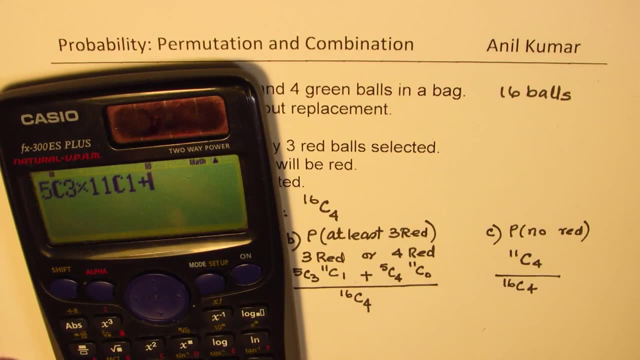 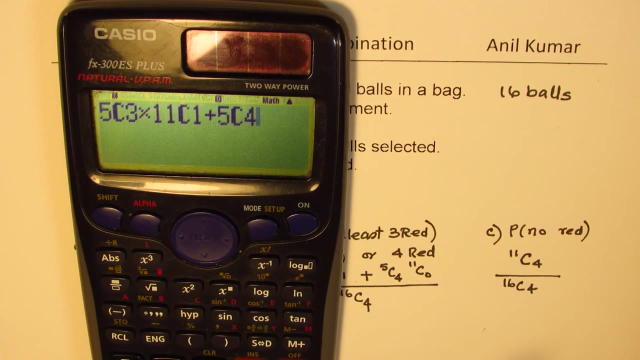 3 times 11, combination 1. plus we have 5 C for 11 C: 0, right all for red. so 5 C 4 times 11 C: 0. so that is the numerator and we are going to divide this by 16 C. 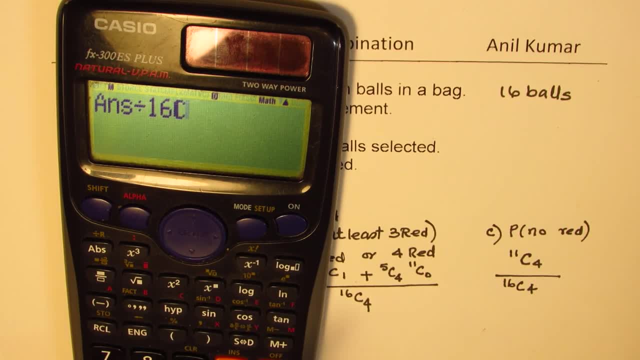 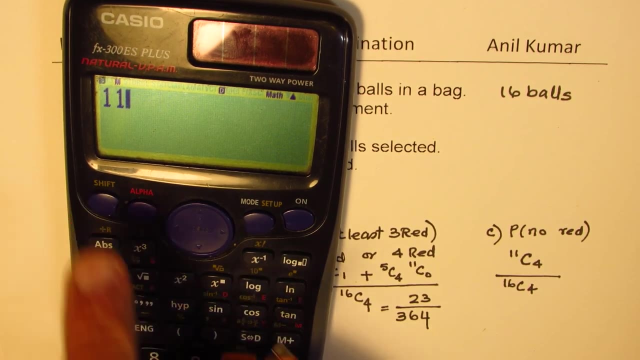 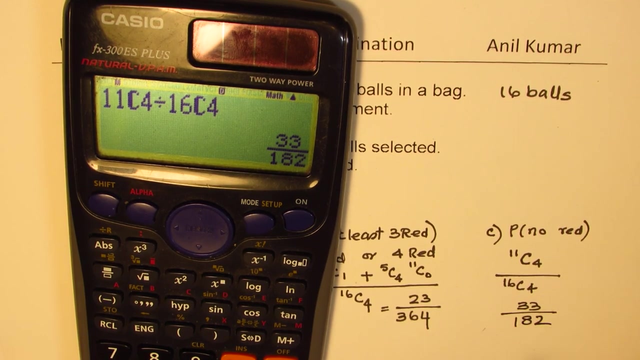 for 16 C 4, right? so that's the answer, which is equal to, in this case, 23 over 364. the last one here: 11 C 4. 11 C 4 divided by 16 C 4, no red balls, is 33 over 182, correct. 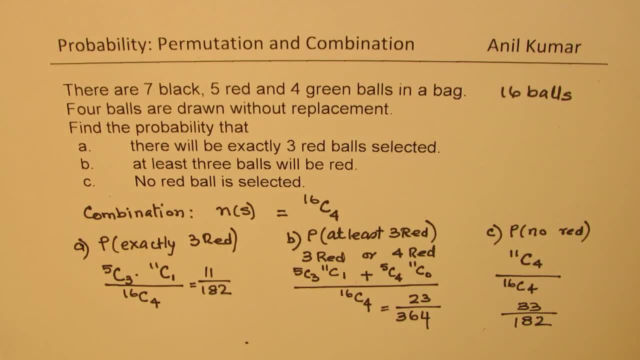 so that's the answer, which is equal to, in this case, 23 over 364. the last one here: 11 C 4. 11 C 4 divided by 16 C 4- no red balls- is 33 over 182, correct? So these are the answers for the three cases. 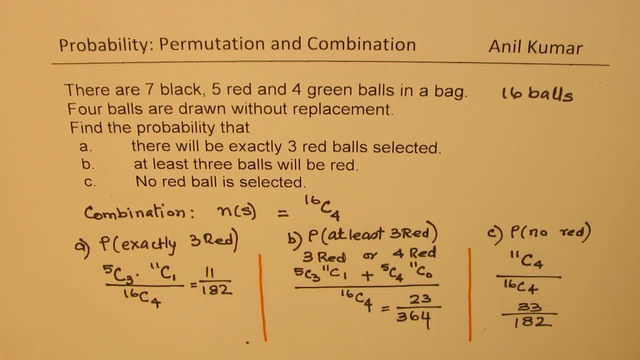 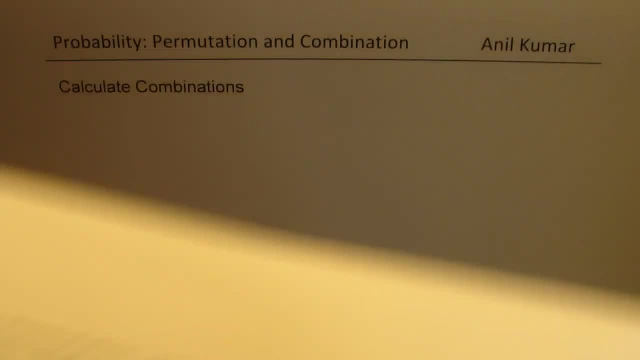 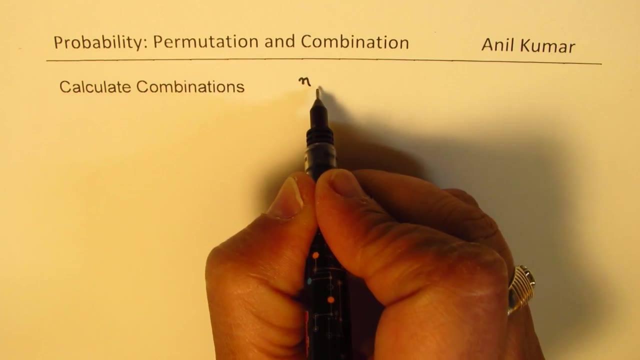 Now we will see how to calculate these values without calculator. Now let's move on to a fresh page to see how to calculate without calculator. So basically we worked out combinations In general. if I have NCR, that means there are N objects and we have to select R out. 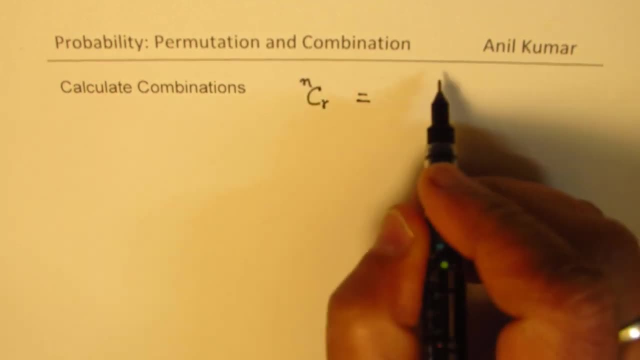 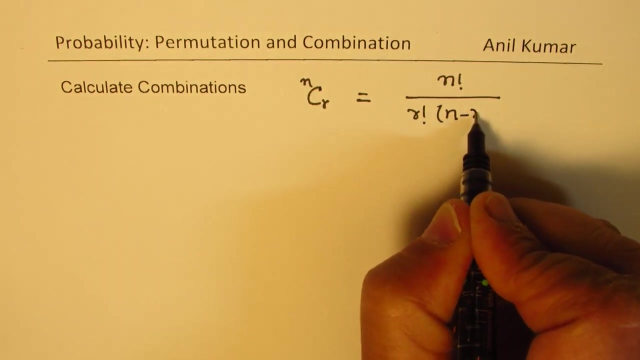 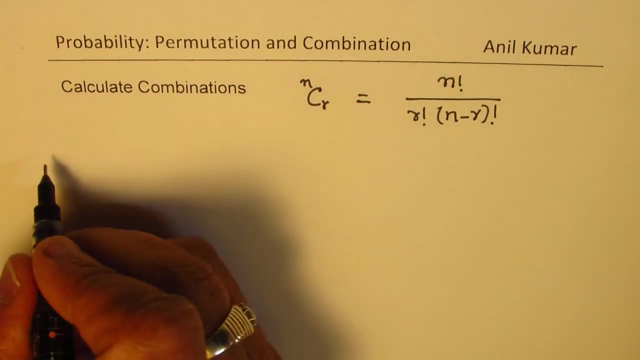 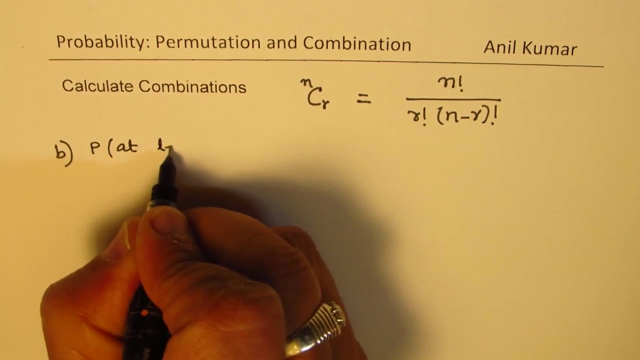 of those objects. In that case the number of combination is N factorial divided by R factorial times N minus R factorial, correct? So in our example we had, let's calculate for one value, let's calculate for B, which was probability for at least three red balls right. 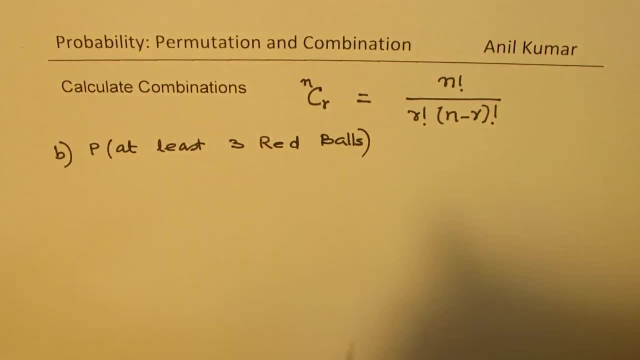 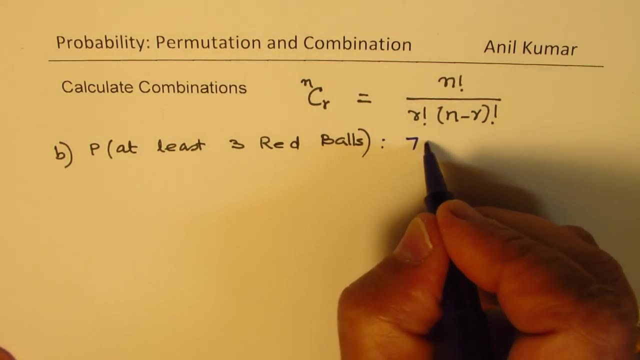 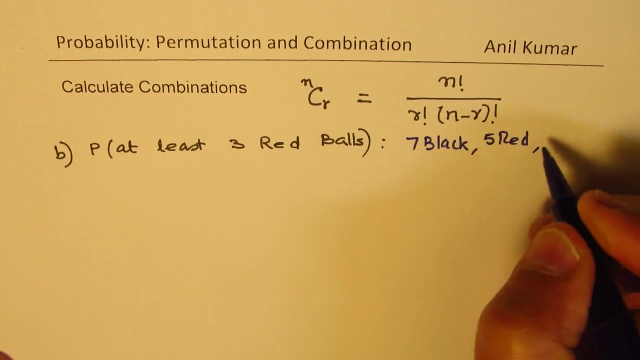 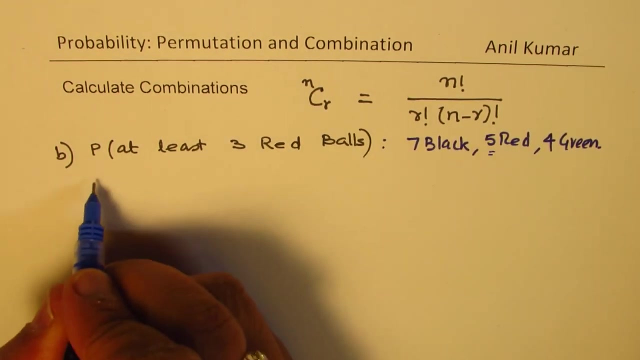 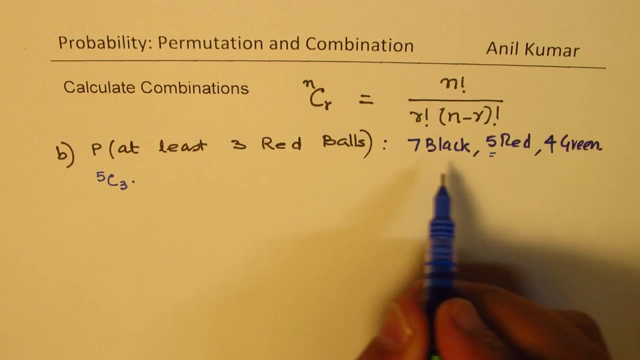 So so we had actually to begin with we had seven black, five red and four green. So if you have to select at least three red balls, then you could, From here, out of these 5, you could select 3.. If you do that, 1 has to be out of 4 and 7, which is 11C1.. Plus, you could select all from the red, so that means 5C4. 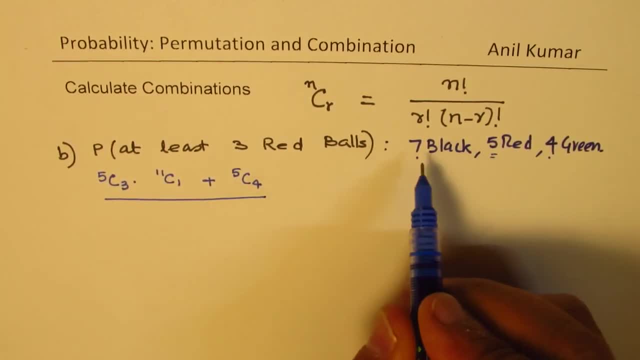 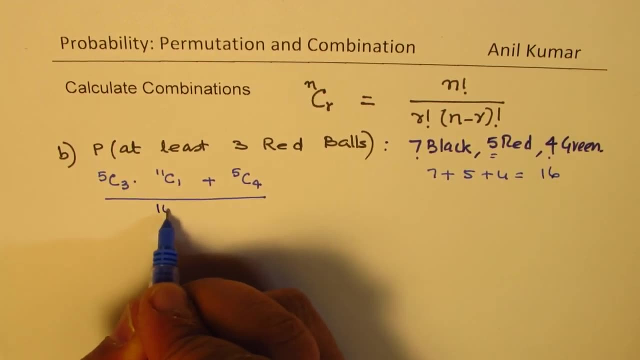 So total number of combinations is, when you add them up, which is 7 plus 5 plus 4, 12 and 4, 16.. So out of 16, we are selecting 4 different balls. So that is what the probability is. 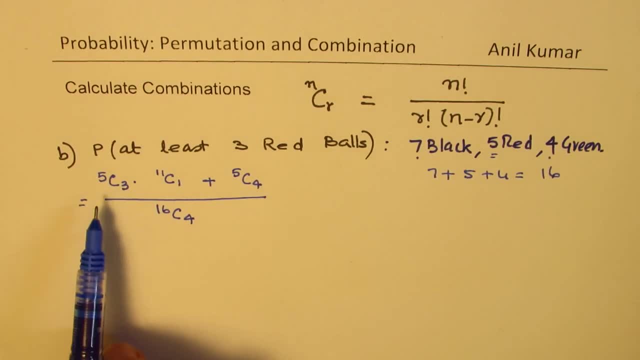 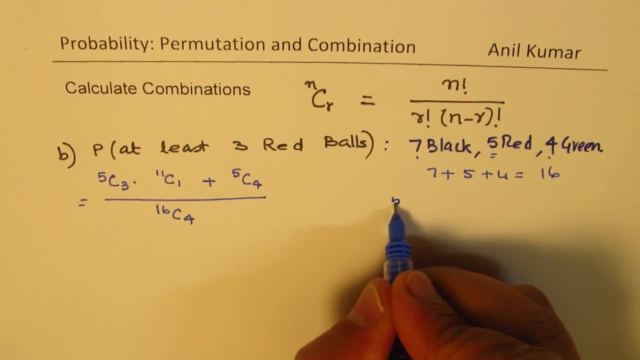 Now the question is how to calculate, correct. So let us calculate these values one by one right, And then we will substitute them there. So when I say 5C3, we will use this particular formula: 5C3.. 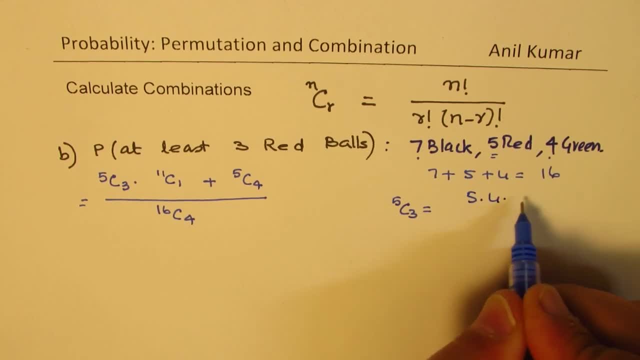 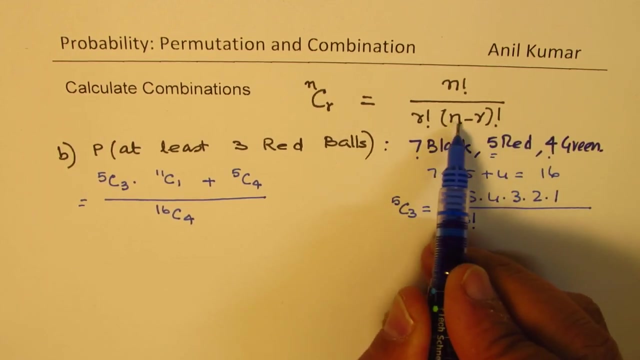 5 factorial means 5 times 4 times 3 times 2 times 1.. That is the meaning of 5 factorial. okay, In the denominator we have r, which is 3 factorial. Let me write 3 factorial. And then we have n minus r, which is 5 minus 3, which is 2 factorial, correct? 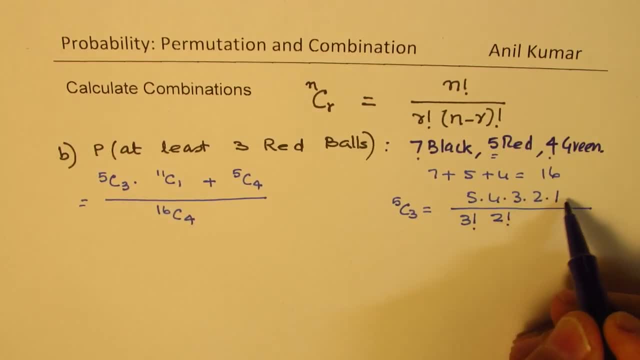 Now 3 factorial basically means 3 times 2 times 1.. So 3 factorial You could cancel with 3 times 2 times 1.. 2 factorial is 2 times 1. So 2 goes 2 times and we get this value as equal to 10, right. 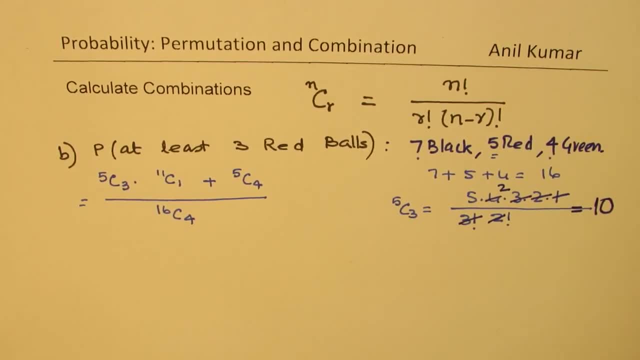 So 5C3 is 10.. Is that clear to you? Now, if I say 11C1,, so that means 11 factorial right, And then we have 1 factorial. 1 factorial is 1.. And then we have 11 minus 1, which is 10 factorial. 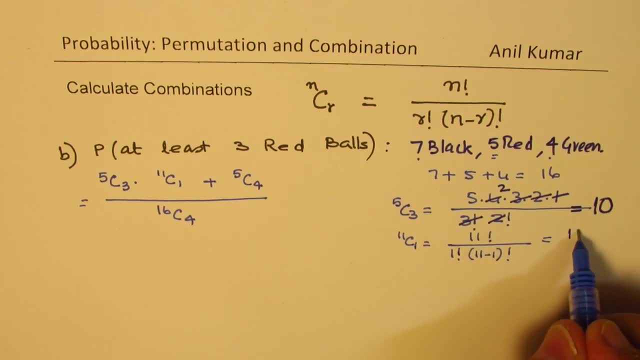 So 11 factorial is 11 times 10 factorial. You're left with 11, only right. So whenever it is 11C1, it will be nC1, will be n. okay, Now the other term is 5C4.. 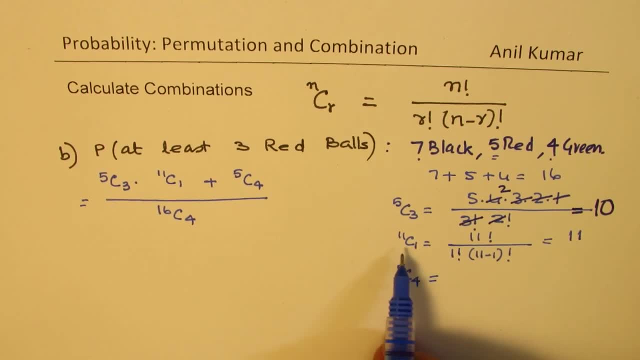 Now, 5C4 is similar to 11C1, and you expect this answer to be 5.. Is that clear to you? You can calculate and then figure this out. Well, the biggest number here to calculate is 6.. 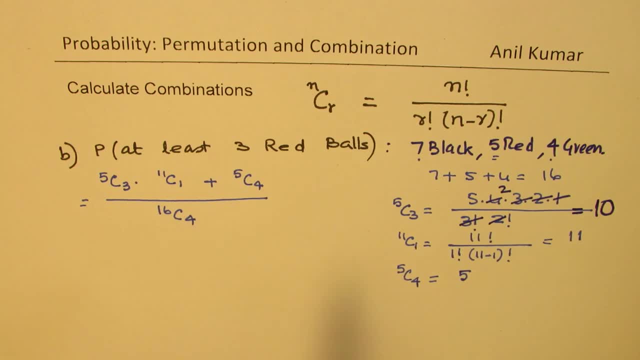 16C4.. So let's see how to calculate 16C4.. So let me just make some room for this So it's not very difficult to calculate, correct? So let's do 16C4 on this side. 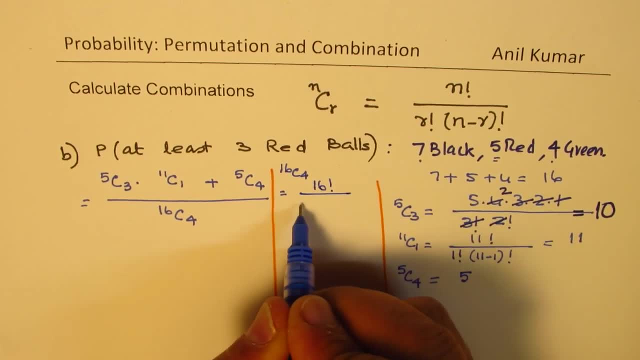 16C4 means 16 factorial over 4 factorial times 16 minus 4, which is 12 factorial. So 12 factorial means We get in the numerator 16 times 15 times 14 times 13 times 12 factorial right. 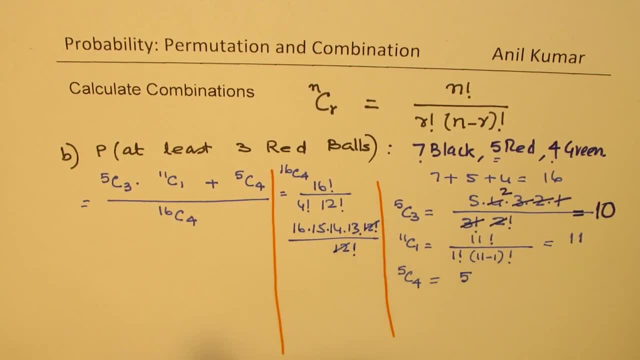 So this 12 factorial cancels with 12 factorial. Do you see that Now we are left with 4 factorial? 4 is 4 times 3 times 2 times 1, okay, So 4 times. 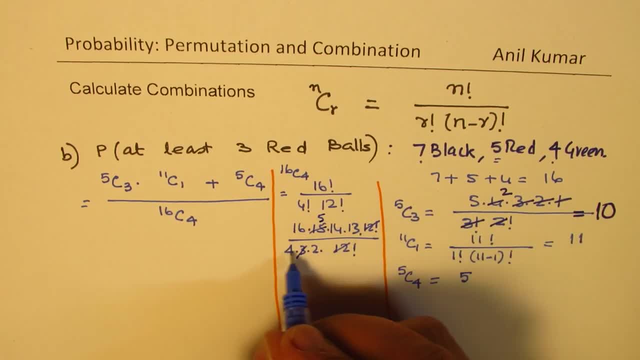 So 3 goes 5 times 4 times 2,, 8 goes 2 times. So we get 14 times 13 times 2 times 5.. Now see 14 times 13,. you could do manually. 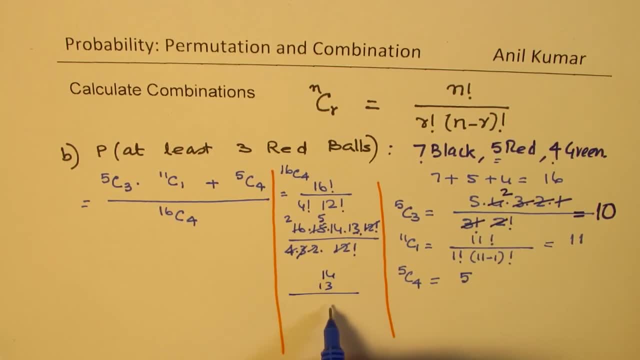 So this is slightly more critical calculation: 3 times 4 is 12, 1. So we get 42 plus 14.. We get 182 times 10. will give you 1820, correct Times 10, which is 5 times 2.. 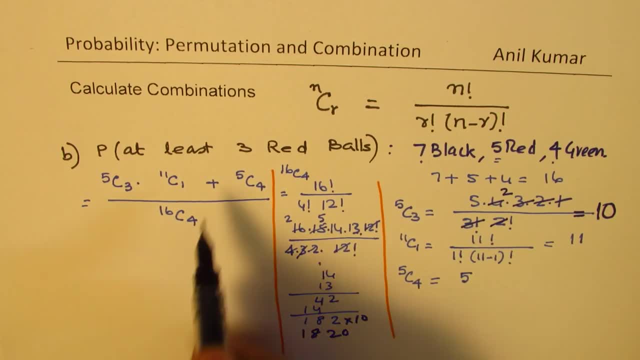 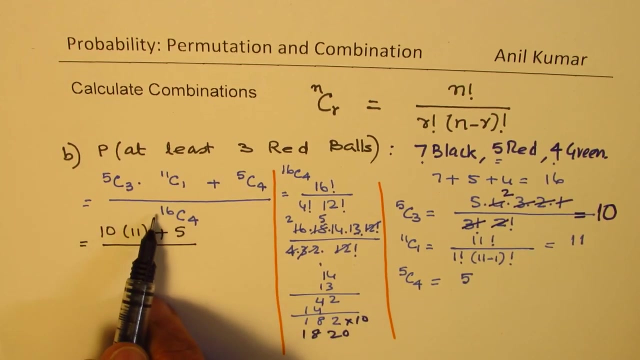 So we have all the numbers here. Let's substitute these numbers and calculate. So 5C3 is 10.. 11C1 is 11 plus 5C4 is 5 and 16C4 is 1820.. 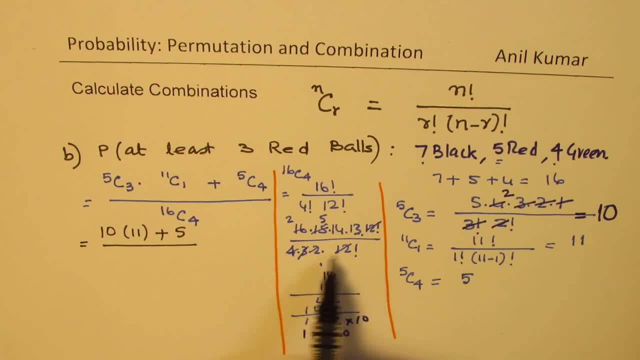 1820 could also be written as it is written. We don't really have to multiply them, right? You will realize why I am saying so Now. I am multiplying, of course. Okay, So this is 110 plus 5.. 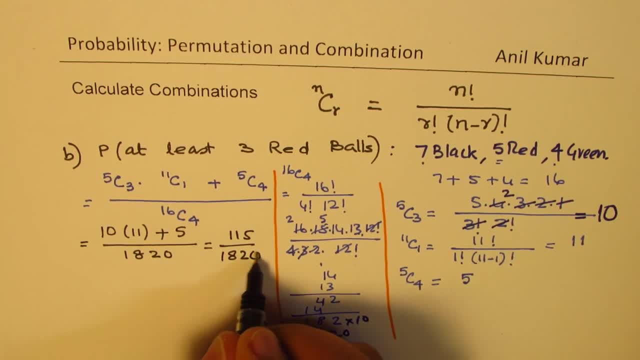 So this is 115 divided by 1820.. Now 5 is common, So let's simplify this: dividing by 5.. 5 times 2 is 10 and 5 times 3 is 15.. Here we get 5 times 3 as 15,, 32,, 6 and 24, right. 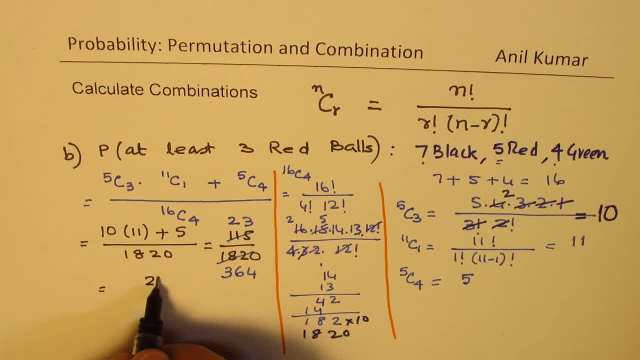 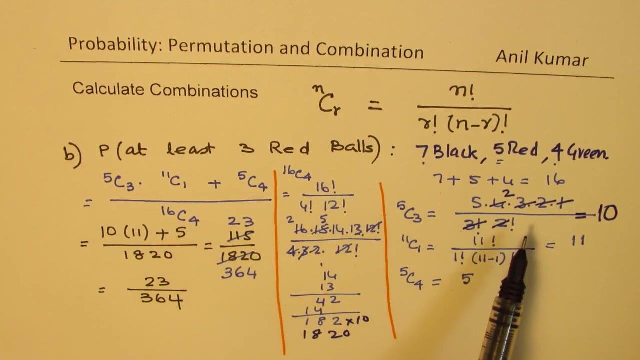 So we get our answer, which is equal to 23 over 364.. So I hope that Steps for calculation is clear to you Now. it looks big amount of calculation when I am showing it here, But once you practice a bit you could directly do it.